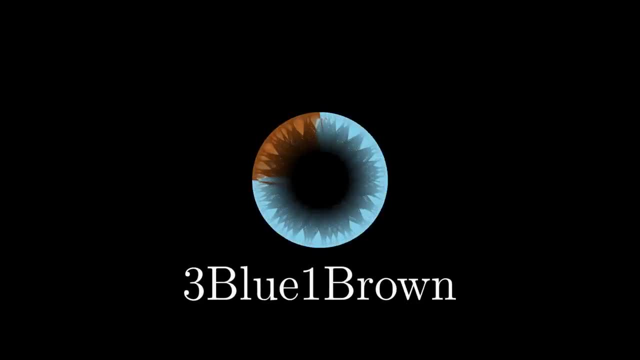 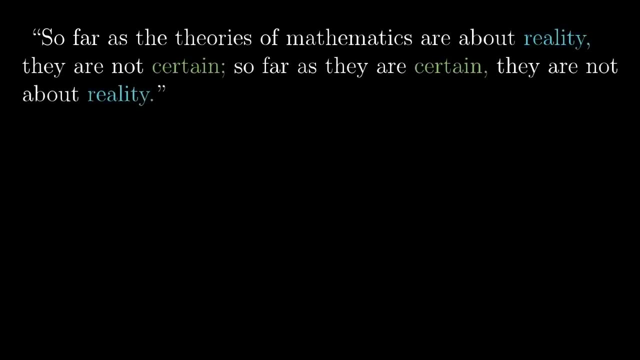 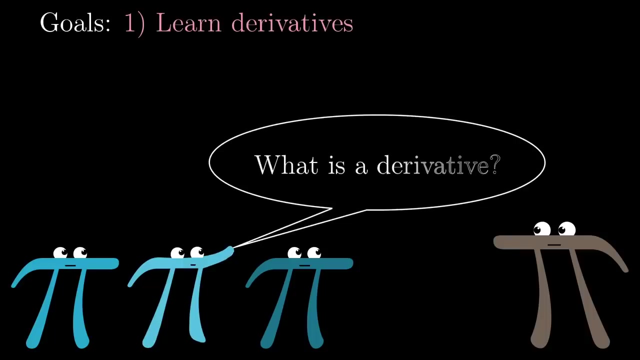 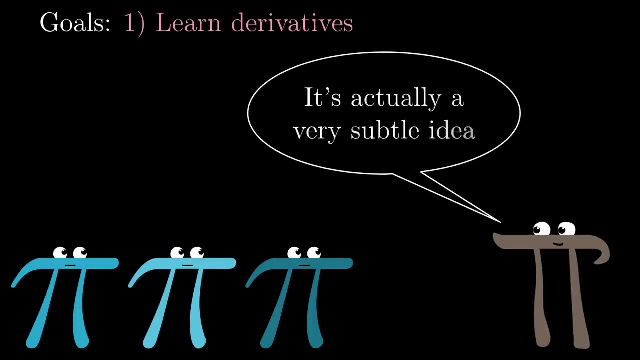 The goal here is simple: Explain what a derivative is. The thing is, though, there's some subtlety to this topic and a lot of potential for paradoxes if you're not careful. So, kind of a secondary goal is that you have an appreciation for what those paradoxes are and how to avoid them. 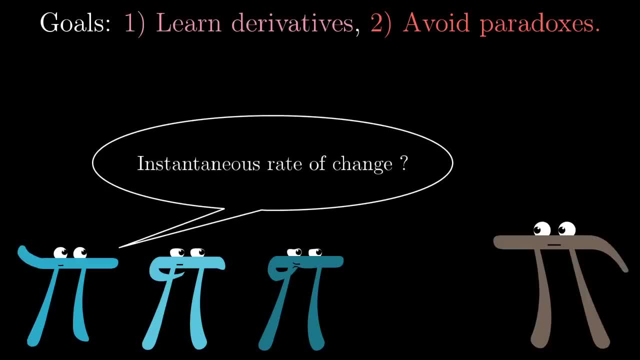 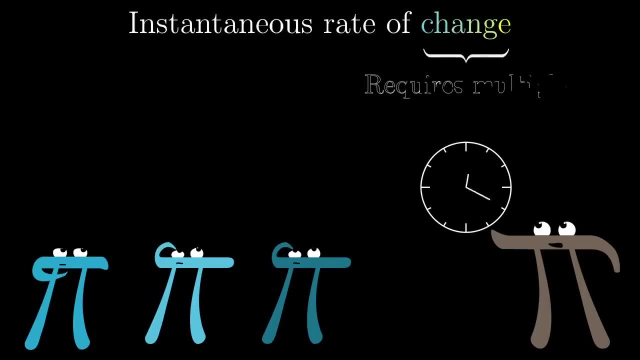 You see, it's common for people to say that the derivative measures an instantaneous rate of change, But when you think about it, that phrase is actually an oxymoron. Change is something that happens between separate points in time and when you blind yourself to all but just a single instant. 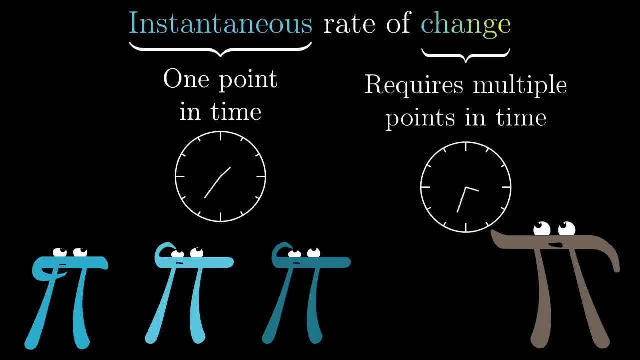 there's not really any room for change. You'll see what I mean more as we get into it. but when you appreciate that a phrase like instantaneous rate of change is actually nonsense, I think it makes you appreciate just how clever the fathers of calculus were. 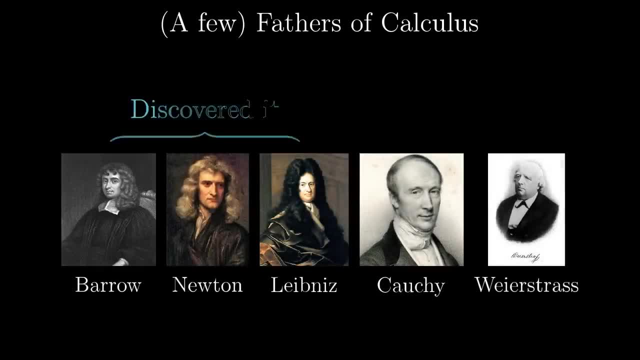 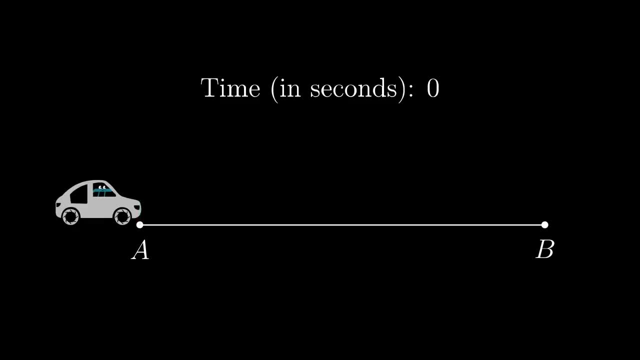 in capturing the idea that that phrase is meant to evoke, but with a perfectly sensible piece of math, the derivative As our central example. I want you to imagine a car that starts at some point A, speeds up and then slows down to a stop at some point B, 100 meters away. And let's say: 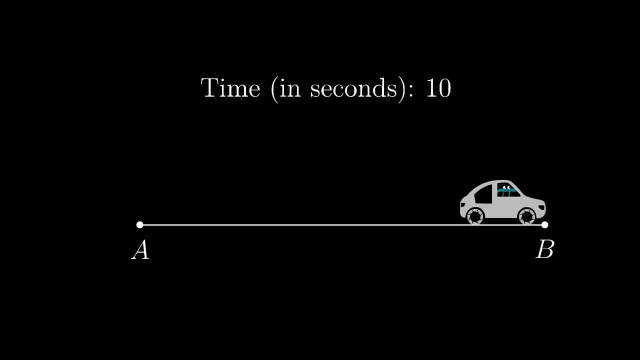 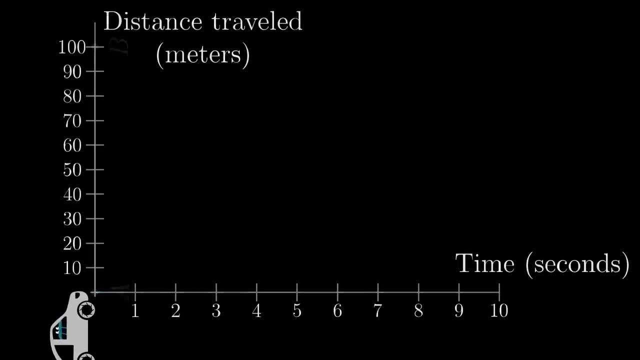 it all happens over the course of 10 seconds. That's the setup to have in mind as we lay out the derivative. So let's start with the first function, letting the vertical axis represent the distance traveled and the horizontal axis represent time. So at each time, t represented with a point somewhere on 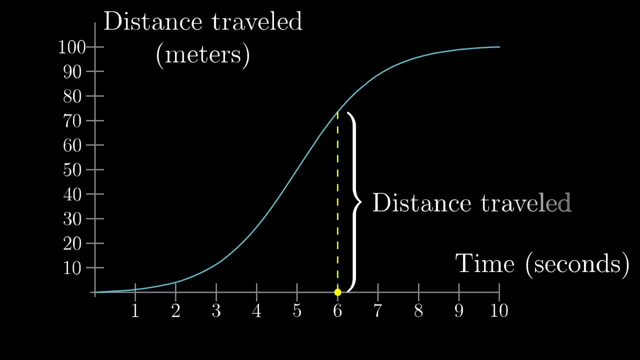 this horizontal axis, the height of the graph, tells us how far the car has traveled in total after that amount of time. It's pretty common to name a distance function like this s I would use the letter d for distance. but that guy already has another full-time job. 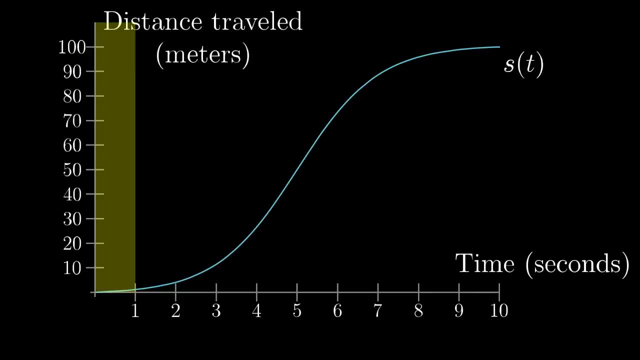 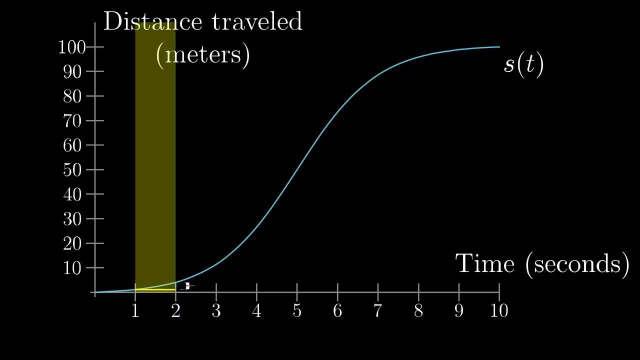 in calculus. Initially this curve is quite shallow. since the car is slow to start, During that first second, the distance that it travels doesn't really change that much. Then, for the next few seconds, as the car speeds up, the distance traveled in a given second gets larger, which 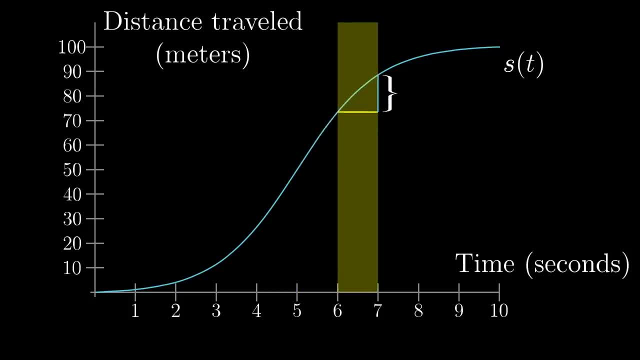 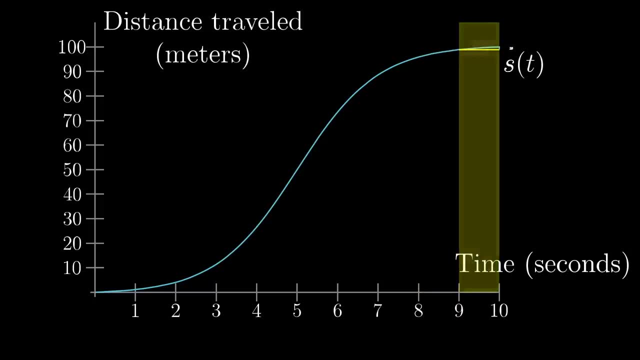 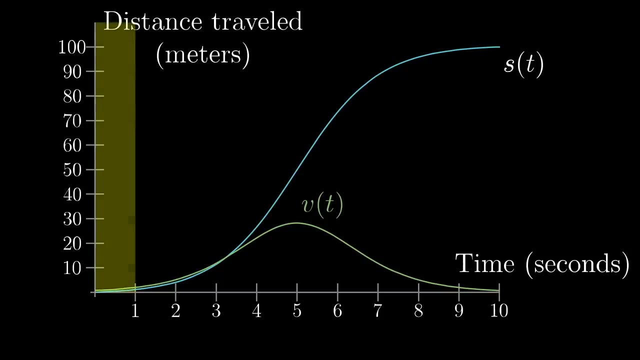 corresponds to a steeper slope in this graph. And then towards the end, when it slows down, that curve shallows out again And if we were to plot the car's velocity in meters per second as a function of time, it might look like this bump. At early times the velocity is very small Up to the middle. 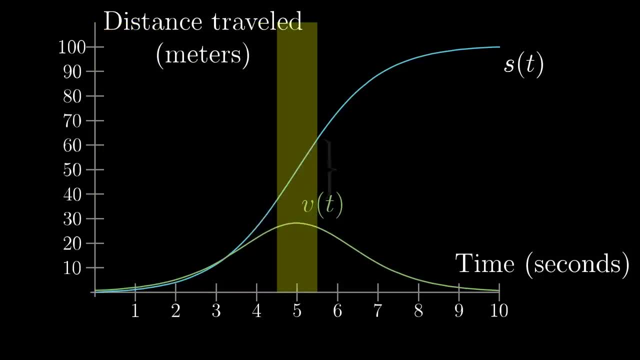 of the journey, the car builds up to some maximum velocity covering a relatively large distance each second. Then it slows back down towards a speed of zero, And these two curves here are definitely related to each other, right, If you change the specific. 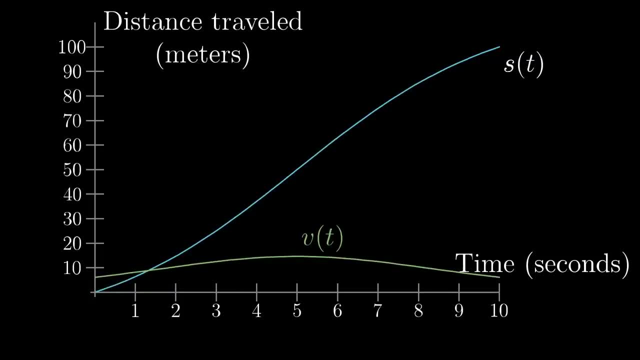 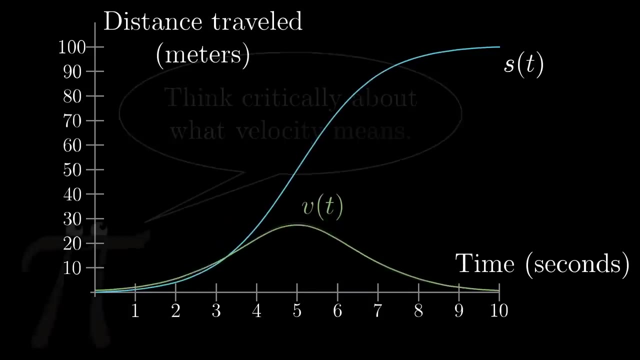 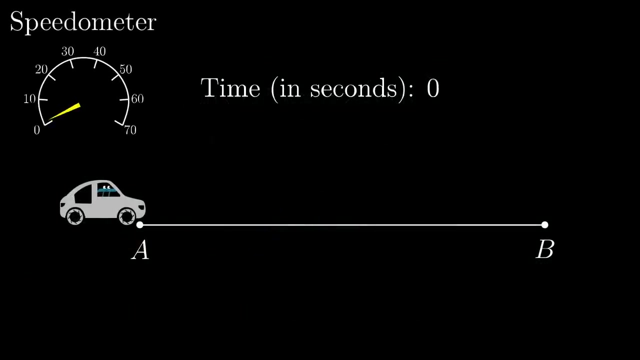 distance versus time function. you're going to have some different velocity versus time function, And what we want to understand is the specifics of that relationship. If we do that, it's worth taking a moment to think critically about what exactly velocity means here. Intuitively, we all might know what velocity at a given moment means. It's just. 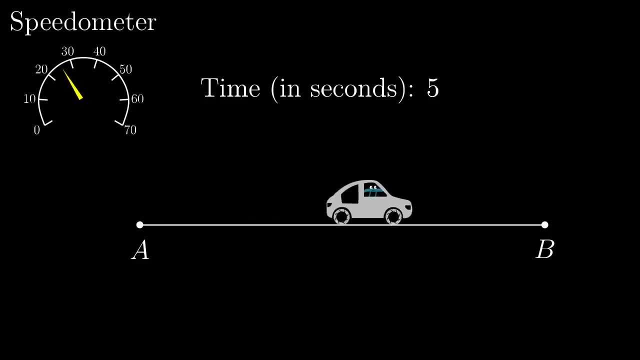 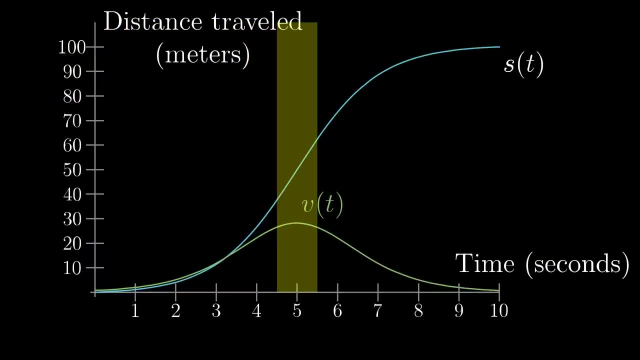 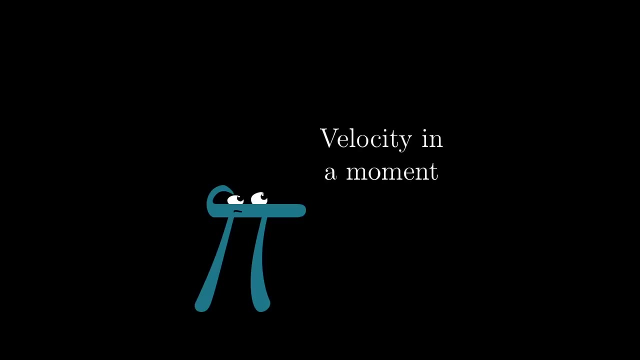 whatever the car's speedometer shows in that moment And intuitively, it might make sense that the car's velocity should be higher at times when this distance function is steeper, when the car traverses more distance per unit time. But the funny thing is, velocity at a single moment makes no sense. If I show you a picture. 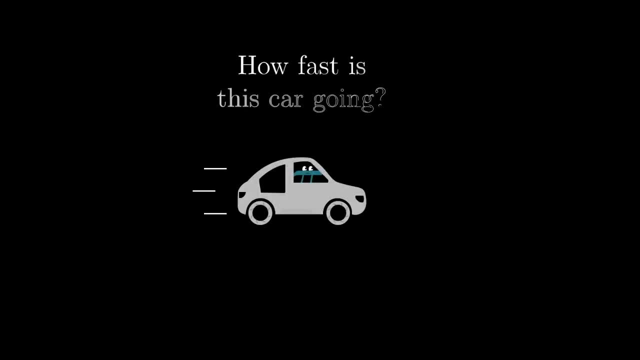 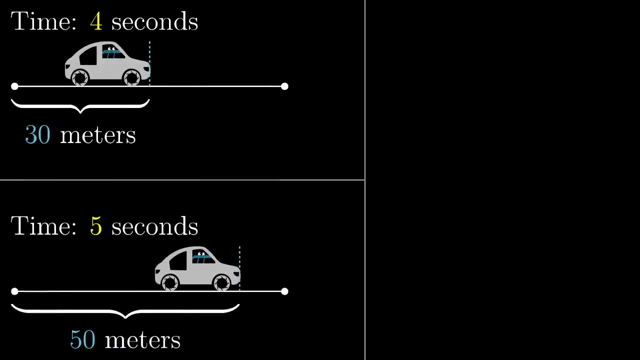 of a car, just a snapshot in an instant, and I ask you how fast it's going. you'd have no way of telling me. What you'd need are two separate points in time to compare. That way you can compute whatever the change in distance across those times is divided by. 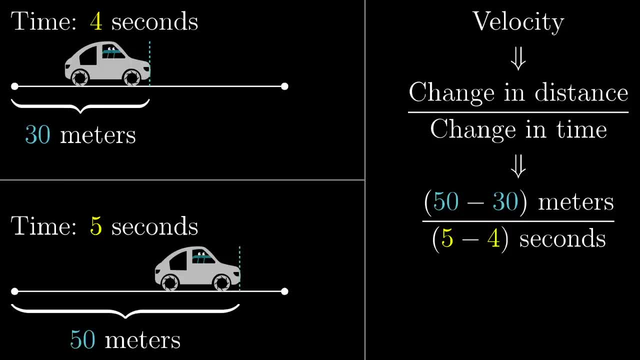 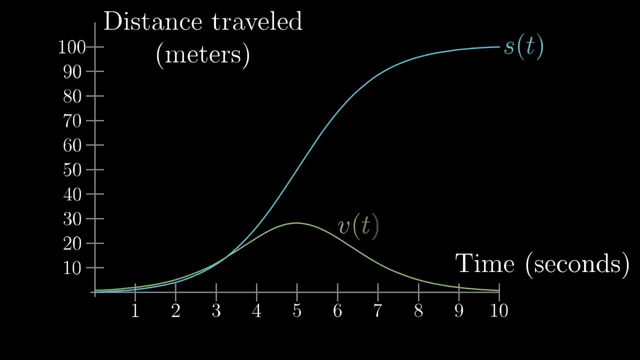 the change in time, Right, I mean, that's what velocity is? It's the distance traveled per unit time. So how is it that we're looking at a function for velocity that only takes in a single value of t, a single snapshot in time? It's weird, isn't it? We want to associate individual. 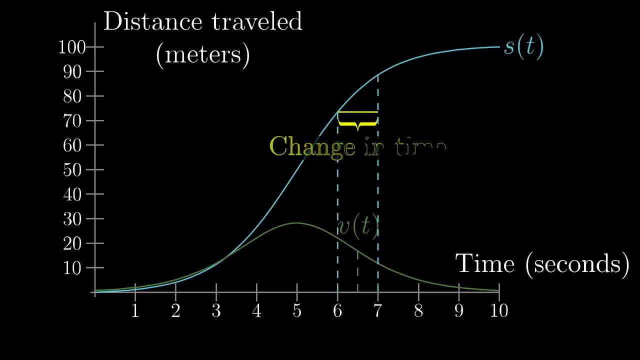 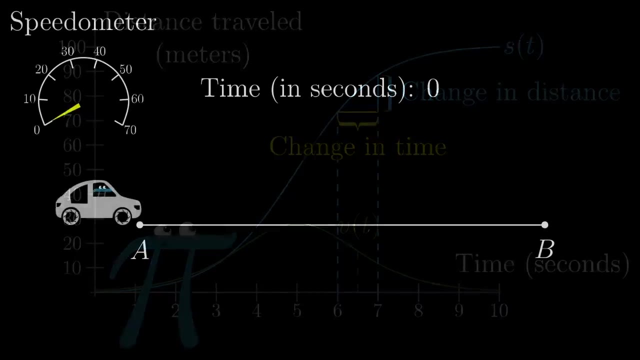 points in time with a velocity. but actually computing velocity requires comparing two separate points in times. If that feels strange and paradoxical, good, You're grappling with the same conflicts that the fathers of calculus did. And if you want a deep understanding for rates of change, 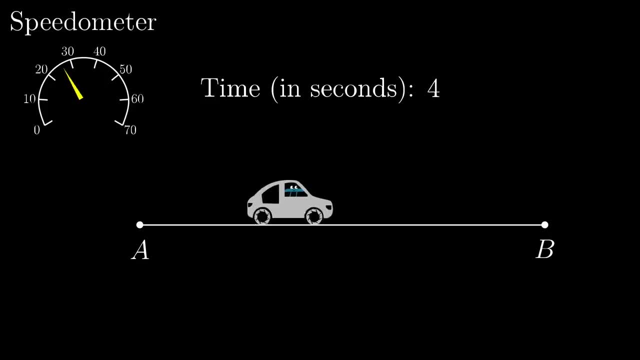 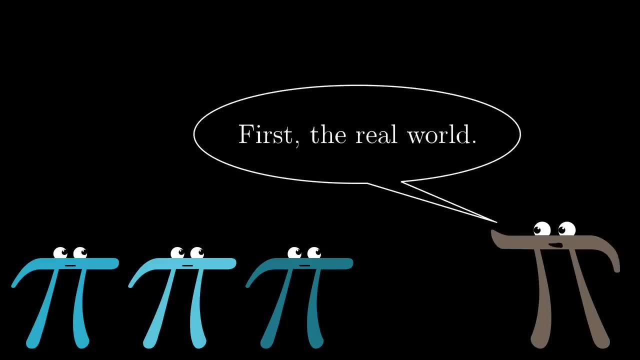 not just for a moving car, but for any car- then you need to know that velocity at a given time is actually a constant. First, I think it's best to talk about the real world and then we'll go into a purely mathematical one. Let's think about what the car's speedometer is probably doing At some. 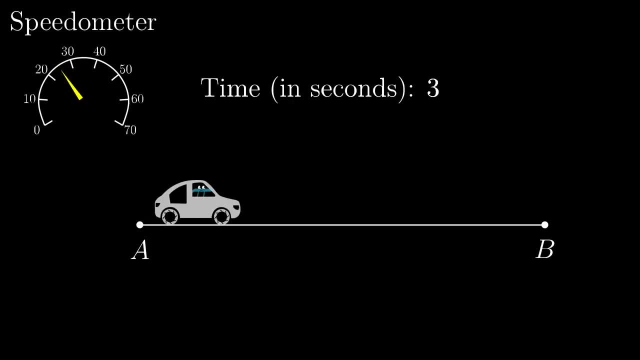 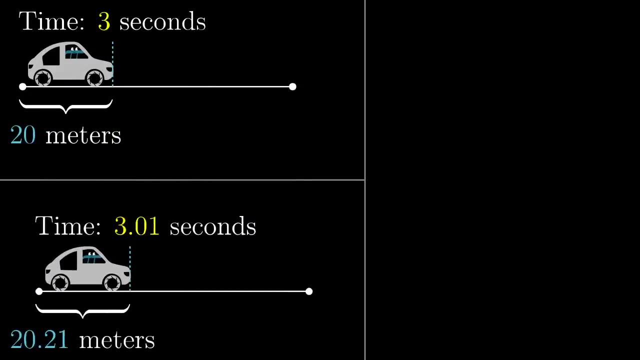 point, say 3 seconds into the journey, the speedometer might measure how far the car goes in a very small amount of time. maybe the distance traveled between 3 seconds and 3.01 seconds. Then it could compute the speed in meters per second. 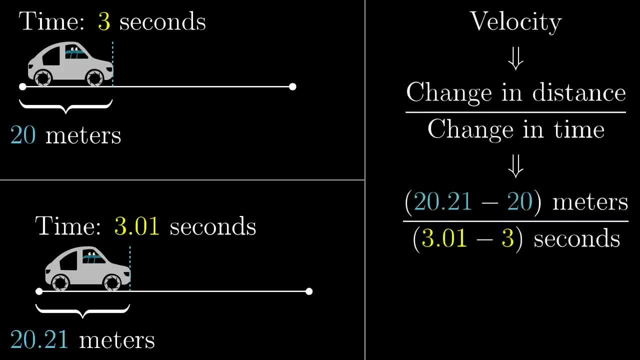 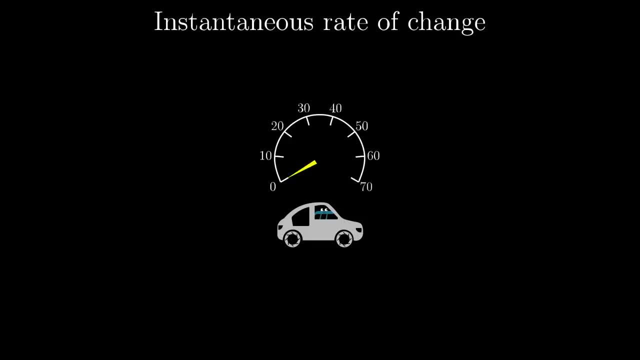 in meters per second, as that tiny distance traversed in meters divided by that tiny time, 0.01 seconds, That is, a physical car just sidesteps the paradox and doesn't actually compute speed at a single point in time. It computes speed during a very small amount of time. 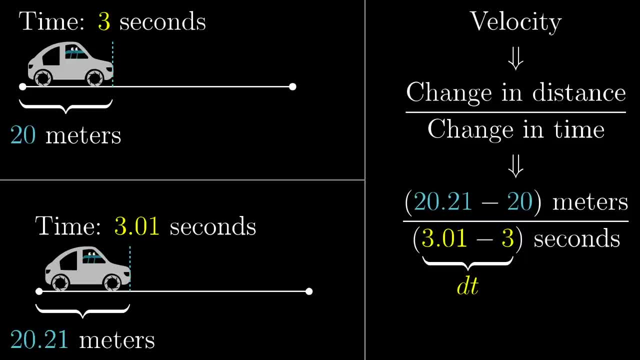 So let's call that difference in time dt, which you might think of in this case as 0.01 seconds, and let's call that resulting difference in distance ds. So the velocity at some point in time is ds divided by dt: the tiny change in distance over the tiny change in time. 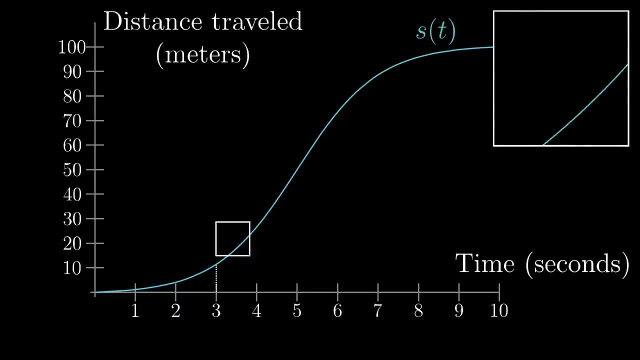 Graphically, you can imagine zooming in on some point of this distance versus time graph. above t equals three. That dt is a small step to the right, since time is on the horizontal axis, And that ds is the resulting change in the height of the graph. 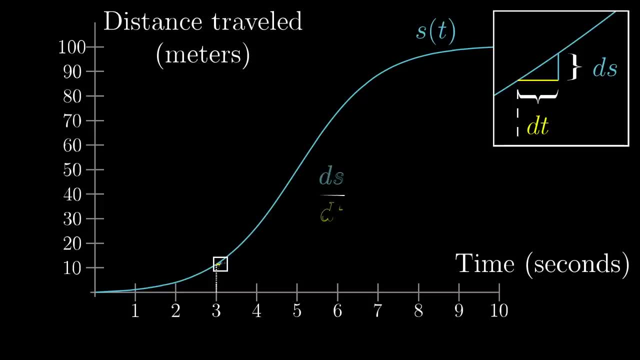 since the vertical axis represents the distance traveled. So ds divided by dt is something you can think of as the rise over run slope between two very close points on this graph. Of course, there's nothing special about the value: t equals three. We could apply this to any other point in time. 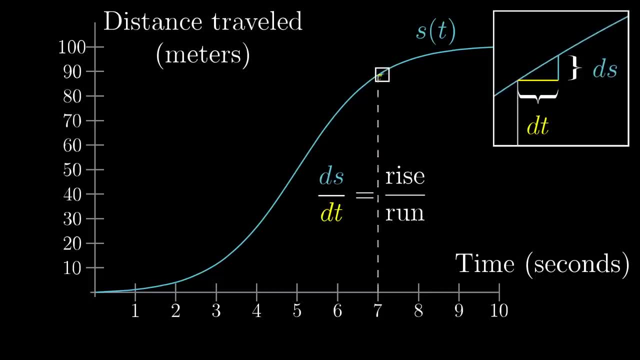 So we consider this expression ds over dt to be a function of t, something where I can give you a time t and you can give me back the value of this ratio at that time, the velocity as a function of time. So, for example, when I had the computer, 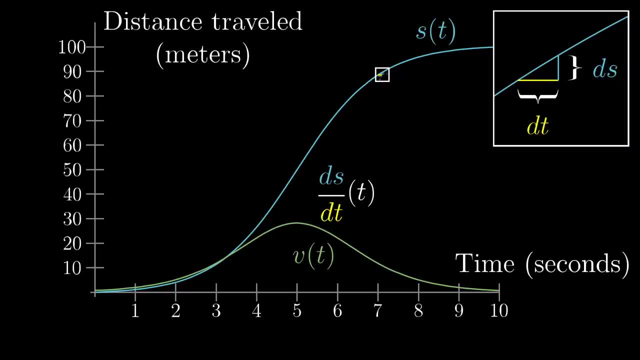 draw this bump curve here representing the velocity function. here's what I had the computer actually do. First I chose a small value for dt, I think in this case it was 0.01.. Then I had the computer look at a whole bunch of times t. 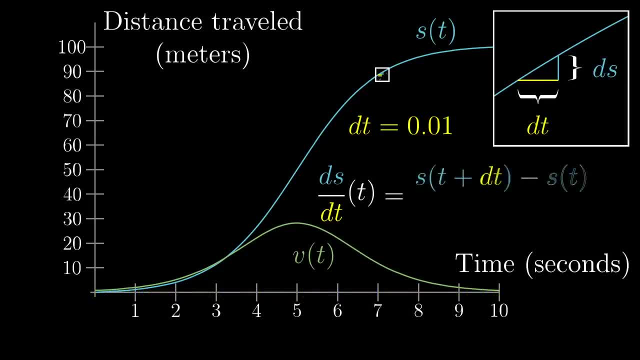 between zero and 10, and compute the distance function s at t plus dt and then subtract off the value of that function at t. In other words, that's the difference in the distance traveled between the given time, t, and the time 0.01 seconds after that. 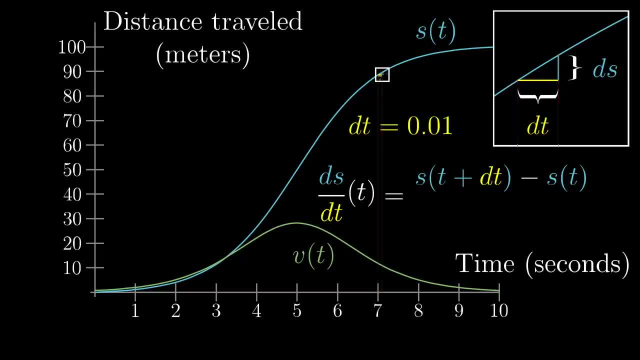 Then you can just divide that difference by the change in time, dt, and that gives you velocity in meters per second around each point in time. So with a formula like this you could give the computer any curve representing any distance. function s of t. 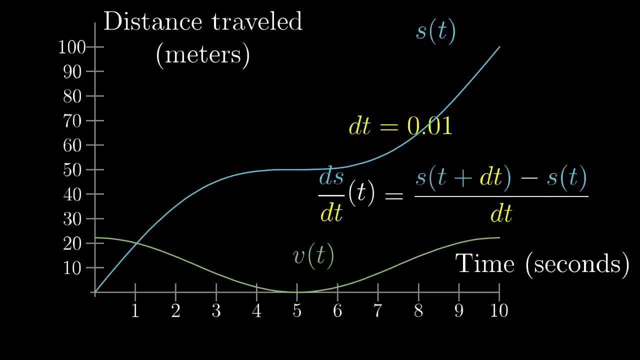 and it could figure out the curve representing velocity. So now would be a good time to pause, reflect, make sure that this idea of relating distance to velocity by looking at tiny changes makes sense, because what we're gonna do is tackle the pattern. 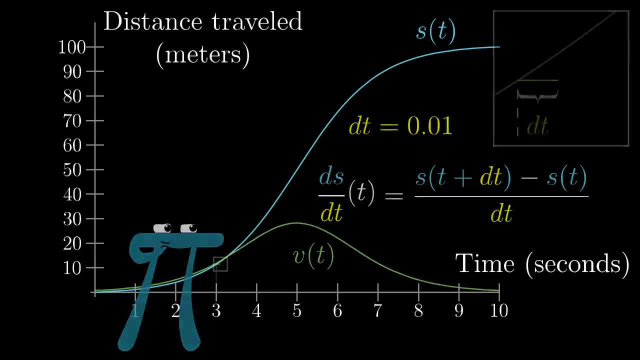 the paradox of the derivative head on This idea of ds over dt. a tiny change in the value of the function s divided by the tiny change in the input that caused it. that's almost what a derivative is, And even though a car's speedometer 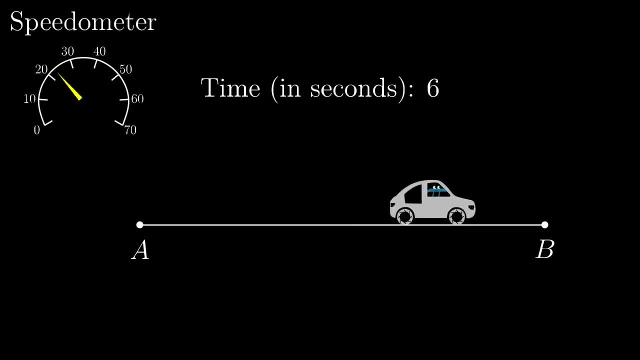 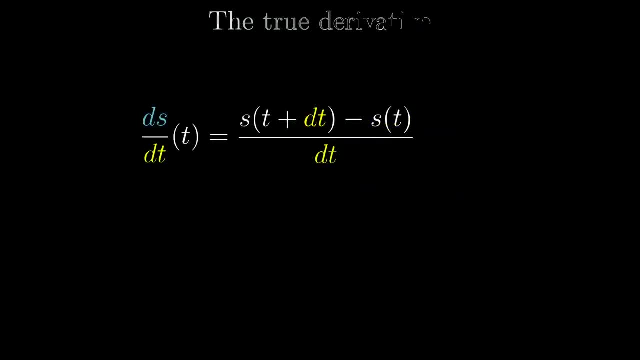 will actually look at a concrete change in time like 0.01 seconds, and even though the drawing program here is looking at an actual concrete change in time, in pure math the derivative is not this ratio: ds, dt for a specific choice of dt. 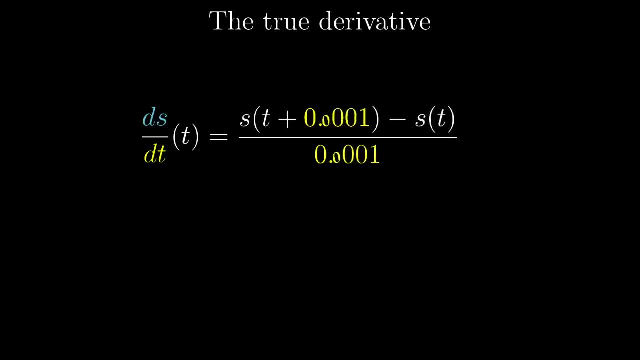 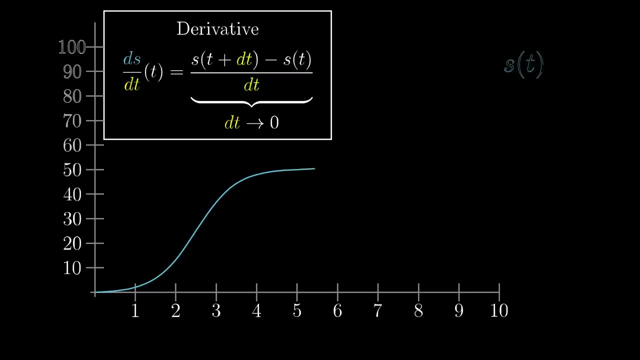 Instead it's whatever that ratio approaches, as your choice for dt approaches zero. Luckily, there is a really nice visual understanding for what it means to ask what this ratio approaches. Remember, for any specific choice of dt, this ratio ds, dt is the slope of a line. 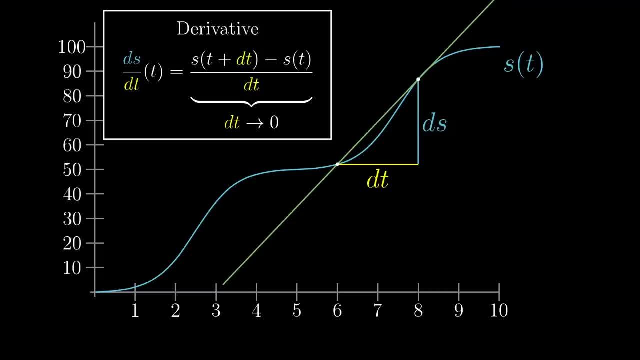 passing through two separate points on the graph right. Well, as dt approaches zero, and as those two points approach each other, the slope of the line approaches the slope of a line that's tangent to the graph, at whatever point t we're looking at. 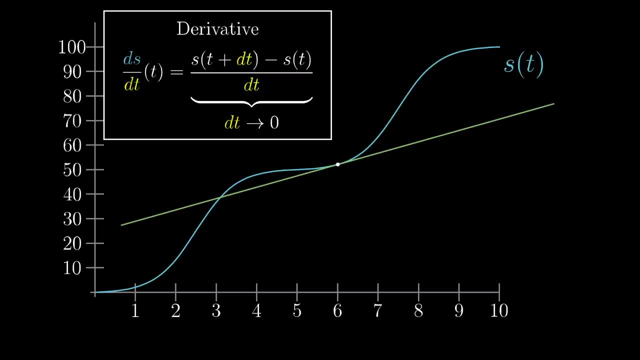 So the true, honest-to-goodness, pure math derivative is not the rise-over-run slope between two nearby points on the graph. it's equal to the slope of a line tangent to the graph at a single point. Now notice what I'm not saying. 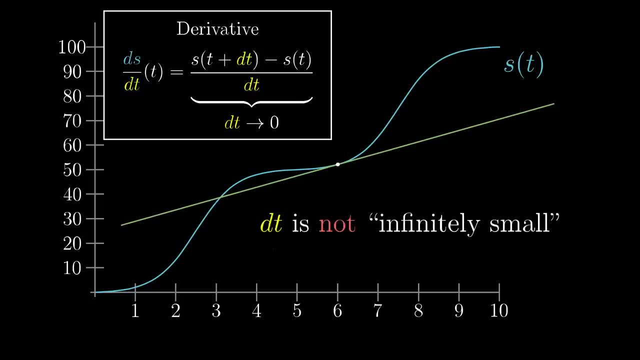 I am not saying that the derivative is whatever happens when dt is infinitely small, whatever that would mean. Nor am I saying that you plug in zero for dt. This dt is always a finitely small, non-zero value. It's just that it approaches zero, is all. 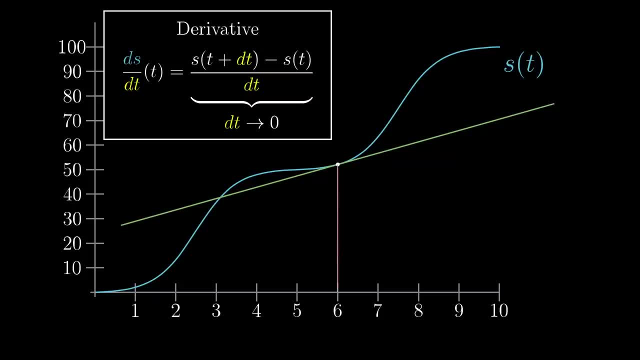 I think that's really clever. Even though change in an instant makes no sense, this idea of letting dt approach zero is a really sneaky backdoor way to talk reasonably about the rate of change at a single point in time. Isn't that neat. 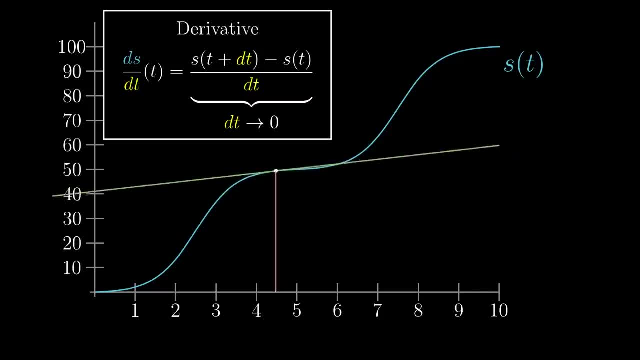 It's kind of flirting with the paradox of change in an instant without ever needing to actually touch it. And it comes with such a nice visual intuition too, as the slope of a tangent line to a single point on the graph. And because change in an instant still makes no sense, 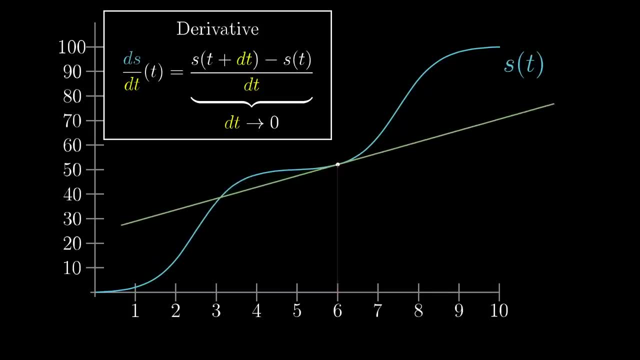 I think it's healthiest for you to think of this slope not as some instantaneous rate of change, but instead as the best constant approximation for a rate of change around a point. By the way, it's worth saying a couple words on notation here. 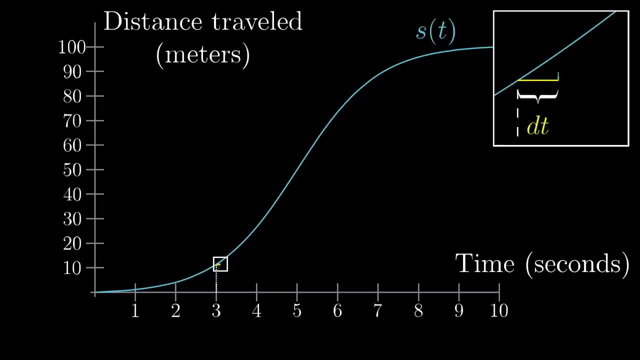 Throughout this video, I've been using dt to refer to a tiny change in t with some actual size, And ds to refer to the resulting change in s, which again has an actual size, And this is because that's how I want you to think about them. 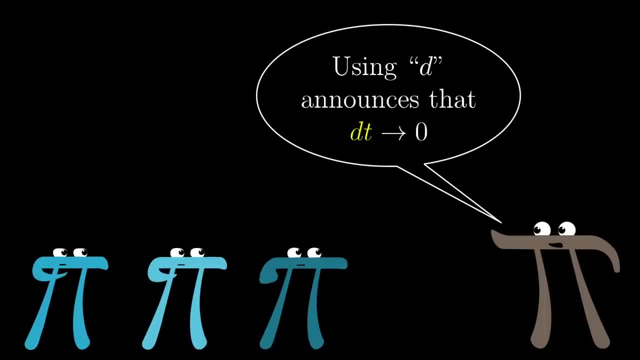 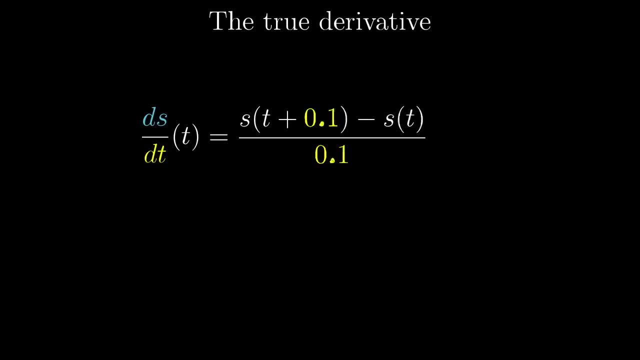 But the convention in calculus is that whenever you're using the letter d like this, you're kind of announcing your intention that eventually you're gonna see what happens as dt approaches zero. For example, the honest-to-goodness pure math derivative is written as ds divided by dt. 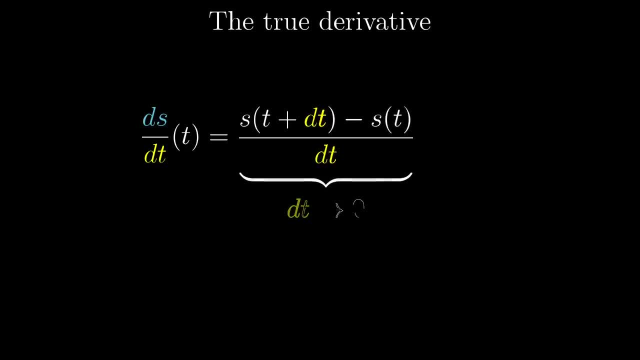 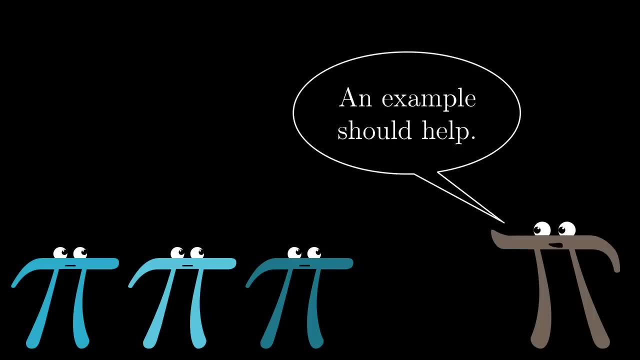 even though it's technically not a fraction per se. but whatever that fraction approaches for smaller and smaller nudges in t, I think a specific example should help here. You might think that asking about what this ratio approaches for smaller and smaller values would make it. 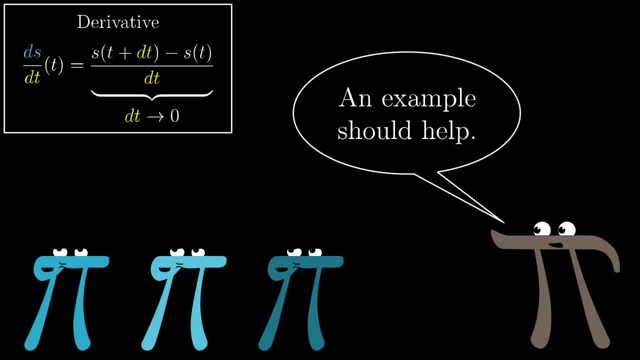 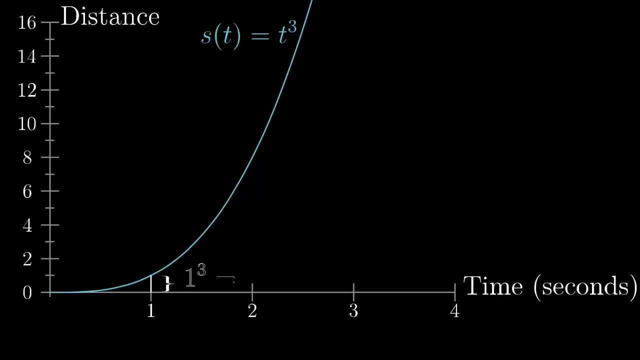 much more difficult to compute, But weirdly it kind of makes things easier. Let's say that you have a given distance versus time function. that happens to be exactly t cubed. So after one second the car has traveled. one cubed equals one meters. 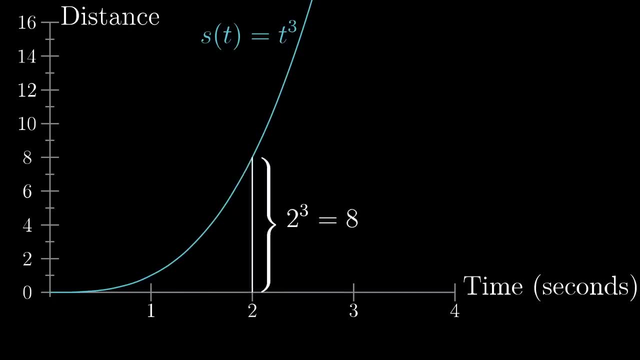 After two seconds it's traveled two cubed or eight meters, and so on. Now, what I'm about to do might seem somewhat complicated, but once the dust settles it really is simpler. and, more importantly, it's the kind of thing. 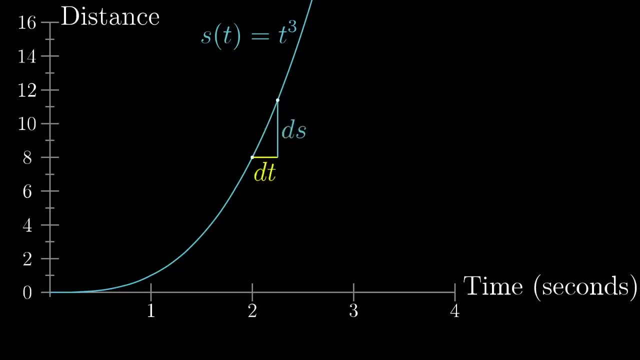 that you only ever have to do once in calculus. Let's say you wanted to compute the velocity ds divided by dt at some specific time, like t equals two, And for right now, let's think of dt as having an actual size, some concrete nudge. 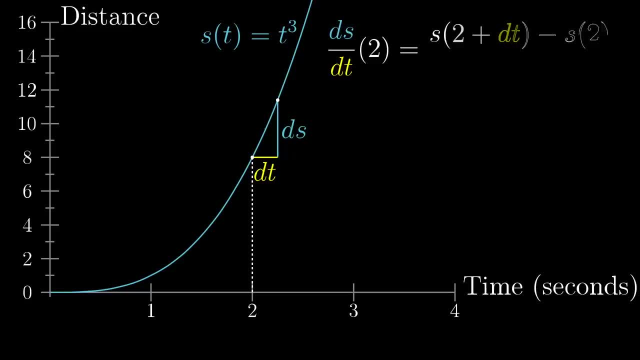 We'll let it go to zero in just a bit. The tiny change in distance between two seconds and two plus dt seconds, while that change is a little bit long seconds. well, that's s of 2 plus dt minus s of 2. And we divide that by dt, Since our 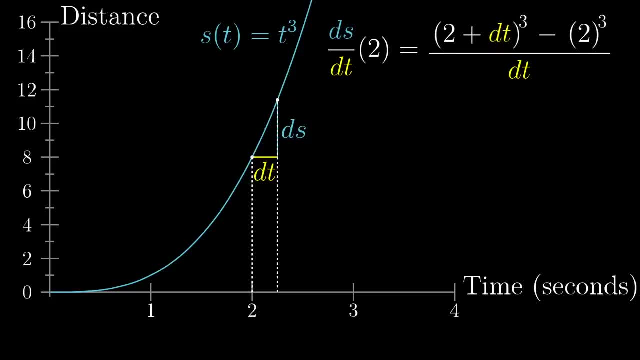 function is t cubed. that numerator looks like 2 plus dt cubed minus 2 cubed. And this, this is something we can work out algebraically. Again, bear with me, there's a reason that I'm showing you the details here. When you expand that top, what you get is 2 cubed plus. 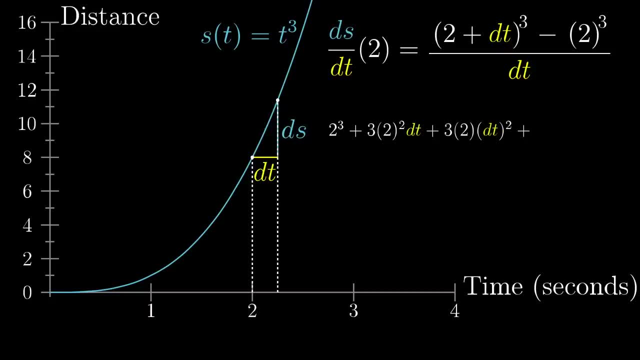 3 times 2 squared dt plus 3 times 2 times dt squared plus dt cubed, and all of that is minus 2 cubed. Now there's a lot of terms and I want you to remember that. it looks like a mess, but it does simplify Those 2 cubed terms. they cancel out And then everything. 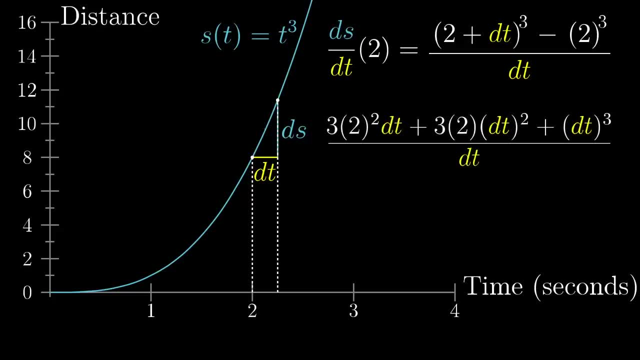 remaining here has a dt in it, and since there's a dt on the bottom there, many of those cancel out as well. What this means is that the ratio ds divided by dt has boiled down into 3 times 2 squared, plus well, two different terms that each. 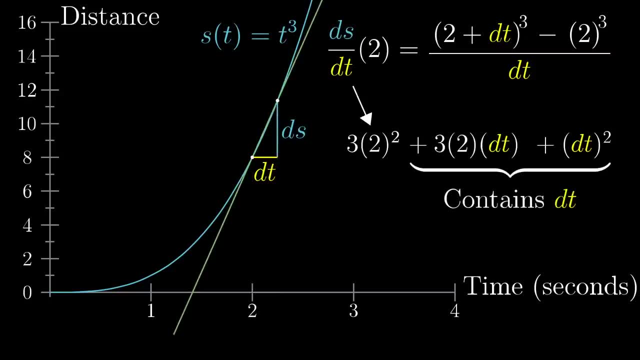 have a dt in them. So if we ask what happens as dt approaches 0, representing the idea of looking at a smaller and smaller change in time- we can just completely ignore those other terms. By eliminating the need to think about a specific dt, we've actually eliminated. 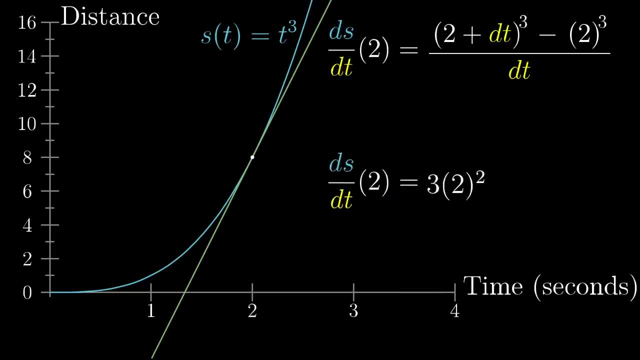 a lot of the complication in the full expression. So what we're left with is this nice, clean, 3 times 2 squared dt. You can think of that as meaning that the slope of a line tangent to the point at t equals 2 of this graph is exactly 3 times 2 squared, or 12.. And, of course, there's nothing. 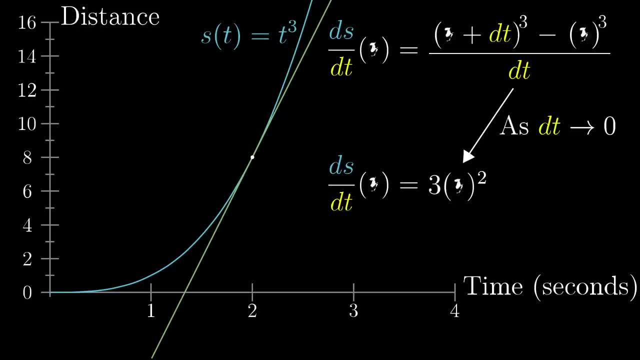 special about the time t equals 2.. We could more generally say that the derivative of t, cubed as a function of t, is 3 times t squared. Now take a step back, because that's beautiful. The derivative is this crazy, complicated idea. 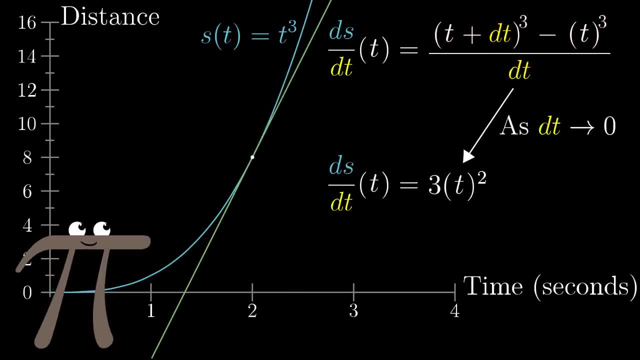 here. We've got tiny changes in distance over tiny changes in time, but instead of looking at any specific one of those, we're talking about what that thing approaches. I mean, that's a lot to think about, And yet what we've come out with is such a simple. 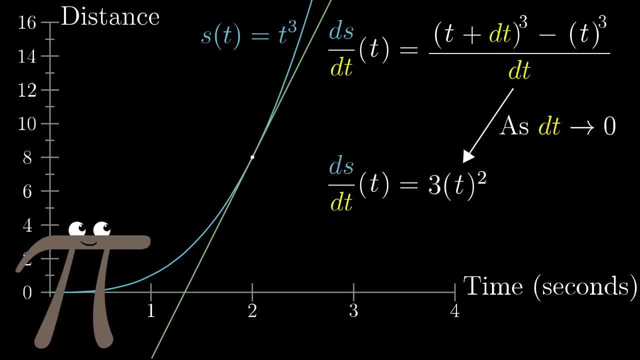 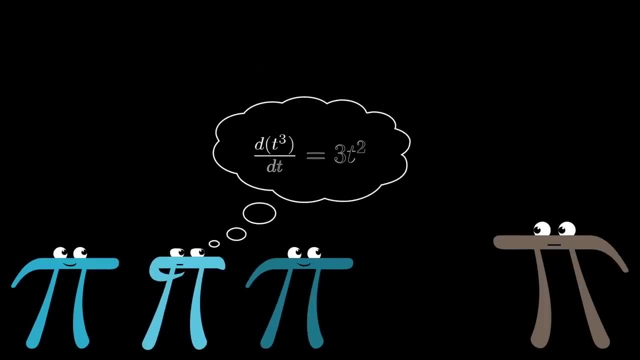 expression 3 times t squared And in practice you wouldn't go through all this algebra each time. Knowing that the derivative of t cubed is 3t squared is one of those things that all calculus students learn how to do immediately, without having to re-derive it each time. And in the next video I'm going. 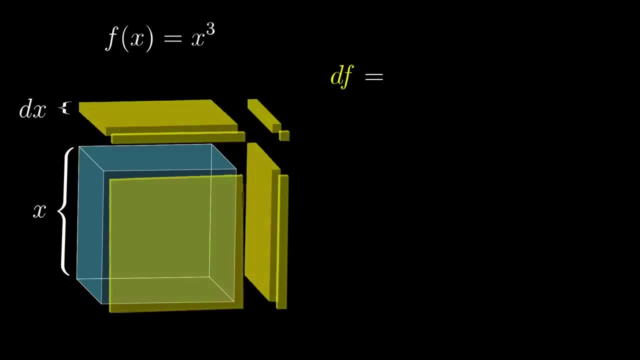 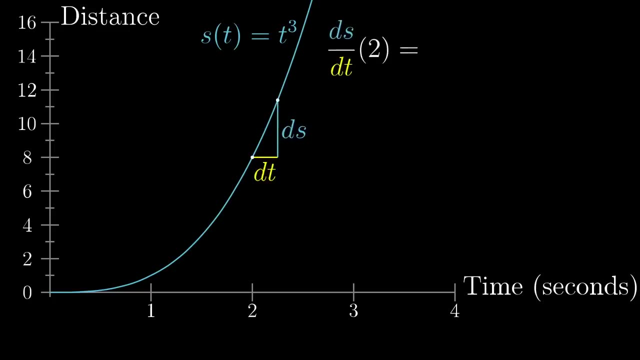 to show you a nice way to think about this and a couple other derivative formulas in really nice geometric ways. But the point I want to make by showing you all of the algebraic guts here is that when you consider the tiny change in distance caused by a tiny change in time for some specific 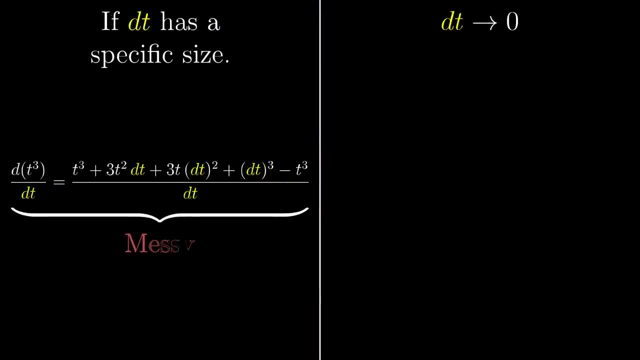 value of dt, you'd have kind of a mess. But when you consider what that ratio approaches- as dt approaches 0, it lets you ignore much of that mess and it really does simplify the problem. That right, there is kind of the heart of why calculus becomes a problem. It's a problem. 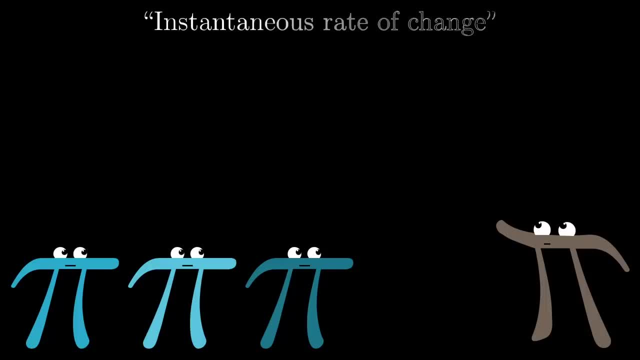 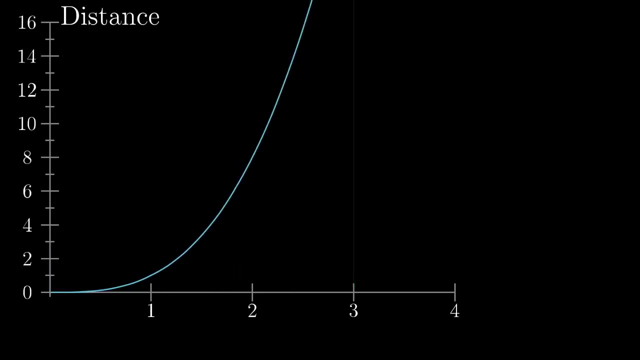 that becomes useful. Another reason to show you a concrete derivative like this is that it sets the stage for an example of the kind of paradoxes that come about if you believe too much in the illusion of instantaneous rate of change. So think about the actual car traveling according to this t cubed distance function and consider. 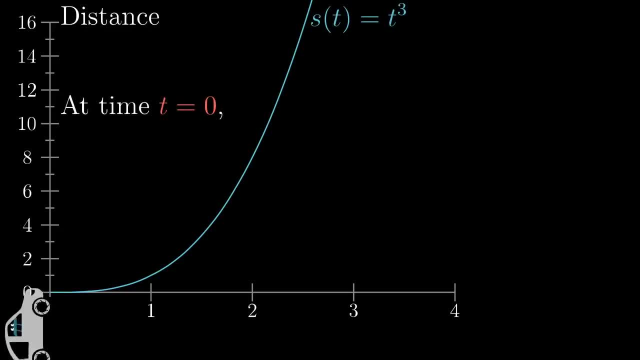 its motion at the moment, t equals 0,, right at the start. Now ask yourself whether or not the car is moving at that time: 1.. On one hand, we can compute its speed at that point using the derivative 3t squared, which: 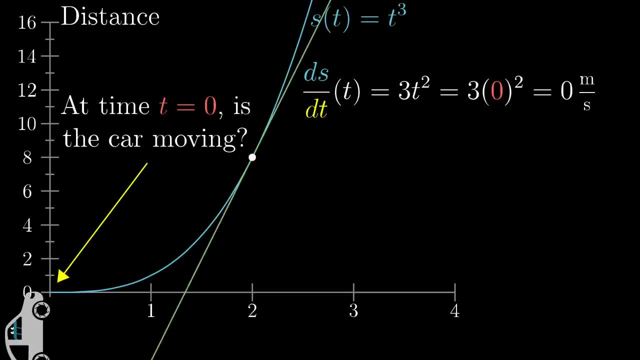 for time t equals 0 works out to be 0.. Visually this means that the tangent line to the graph at that point is perfectly flat. so the car's quote-unquote instantaneous velocity is 0, and that suggests that obviously it's.